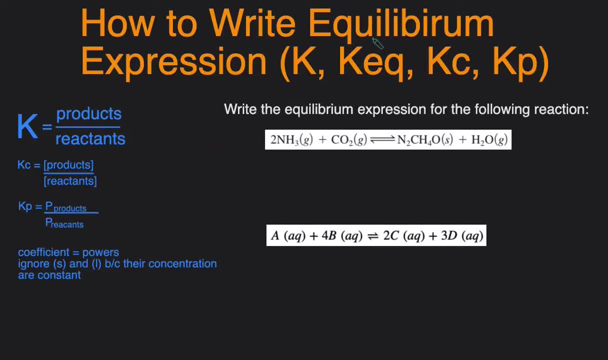 Hey guys, this is Mike from Conquer Chemistry. In today's video we'll be looking at how to write equilibrium constant expressions, k, keq, kc and kp In general. k is the products divided by reactants or products over reactants. If you're asked to write kc, then it'll be concentration of products. 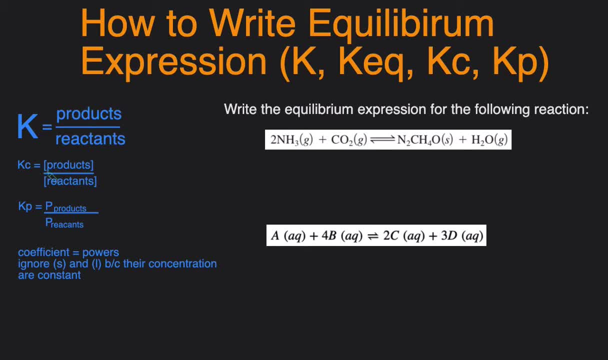 over concentration of reactants. The c right here stands for concentration, and that's what those brackets also stand for. kp is the pressure of products over the pressure of reactants. If you're just asked to write k or keq without the specification of kc and kp, then just default. 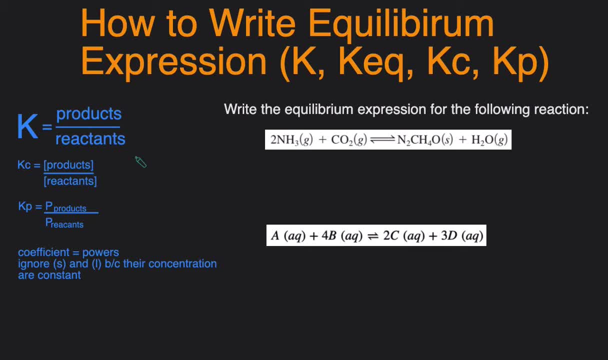 to using concentration, unless otherwise specified. so You might want to also just double check with your teacher, because different teachers have different preferences regarding k and keq. The coefficients in the reaction become the exponents or the powers, and then, lastly, ignore the salts and liquids, because their concentrations are constant. Now let's take a look at a couple. 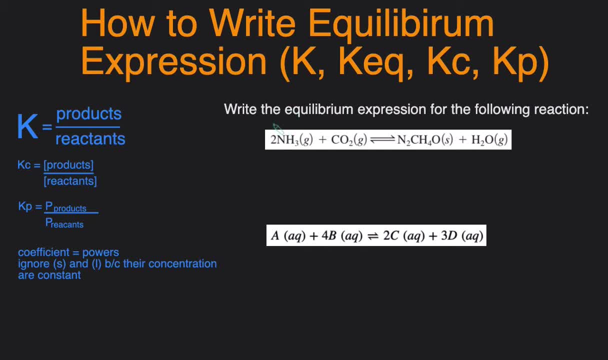 examples to see how these rules are applied. So for these problems, we will be writing the equilibrium constant expressions for the following reactions: For this first reaction, let's start off by looking at the equilibrium constant expression. For this first reaction, let's start off by looking. 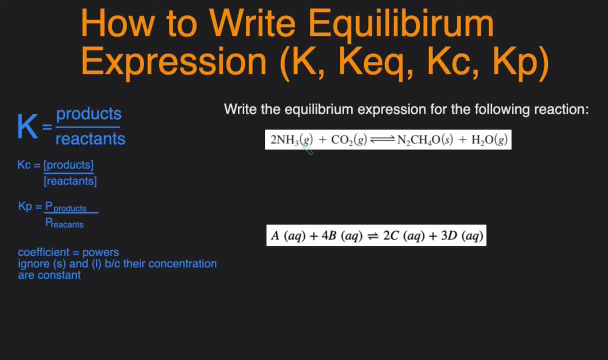 taking a look at the states and just crossing any salts and liquids out, because we ignore those. So we have a gas, a gas solid, cross this out and then a gas. So, since all these are gases, we have the option of writing either kc, expressing it in concentration, or kp. I'll show you both. So kc. 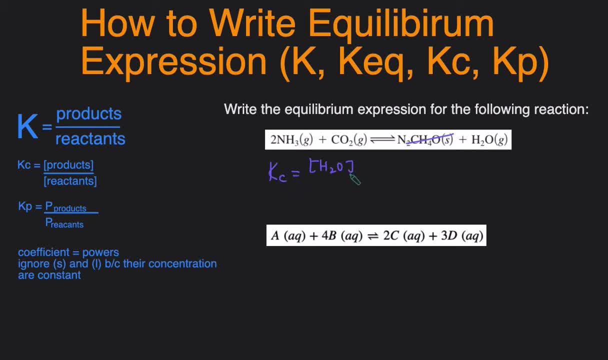 would be the concentration of H2O, raised to the first power, because that's a coefficient of one divided by the concentration of reactants, which is the NH3. raised to the second power because this coefficient multiplied by the concentration of CO2, raised to the first power. For kp, we'll just be using pressure, so be pressure of the products. 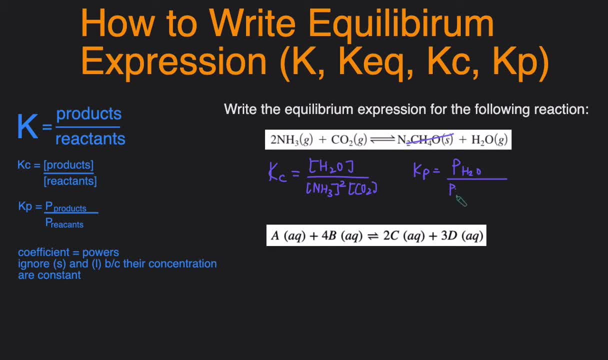 H2O divided by pressure of the reactants, NH3, squared because the coefficient two multiplied by the pressure of CO2.. Next sample: the first thing we'll do is just look at all the states. so aqueous, aqueous, aqueous, aqueous. There's no solid liquids to cancel out, Since all these are. 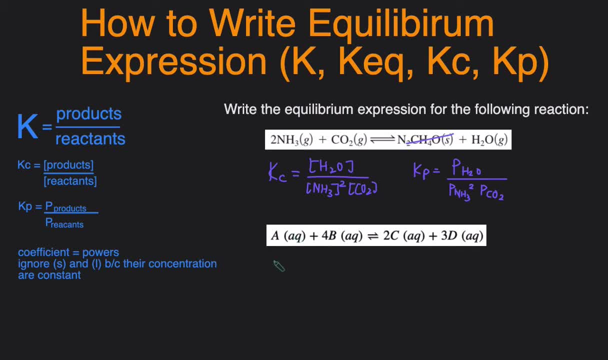 gases, we can only write kc, because then you can only use kp if there are gases. So kc or just k would equal the concentration of the product, c squared because of two, multiplied by d, raised to the third power, divided by the concentration of reactants on the bottom. 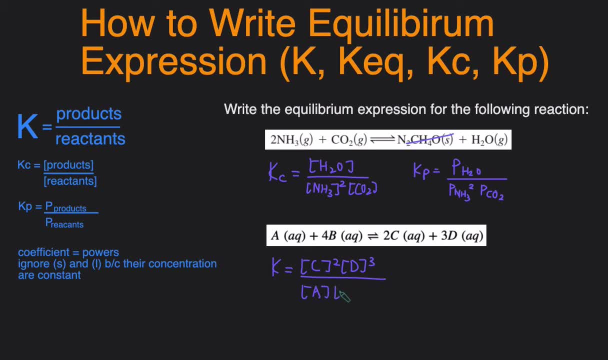 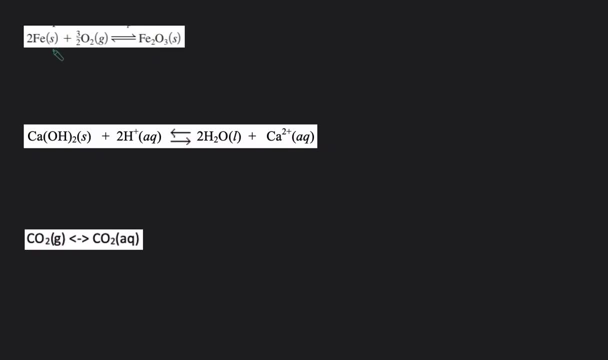 a, raised to the first power, because that's no coefficients, multiplied by b, raised to the power of four, because that's a coefficient of four. The next sample: we'll start again by crossing any solid liquids out. Cross one out, cross one out. and since this is a gas, 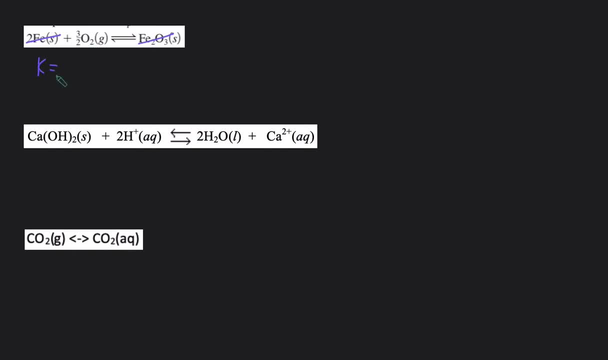 that's left over. we can write kc or kp. We can write k is equal to, and since we have crossed out the product and there's no other product, then we'll just default to using a one here, One divided by the concentration of O2 raised to the power of three over two. or we can also write kp, which is: 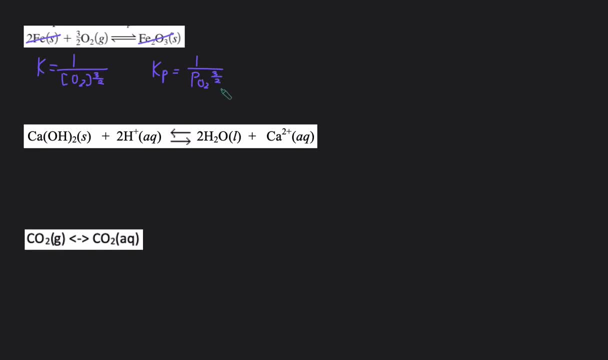 the pressure of O2 raised to the power of 3 over 2.. Next one, again, start off by crossing solids and liquids out. Cross out the solid here and the liquid here. Both of these are aqueous, so we'll use this concentration. k equals the concentration of Ca2 plus divided by the concentration. 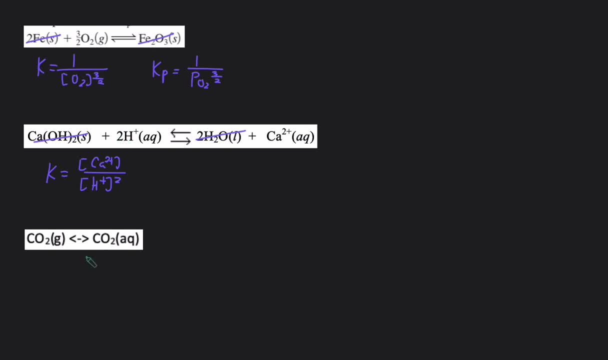 of H plus squared because of the coefficient. Last example: we have both a gas and aqueous here, so typically aqueous is when you use concentration and for gases you have the option of using concentration or pressure, but when you have both in the same reaction, use concentration. 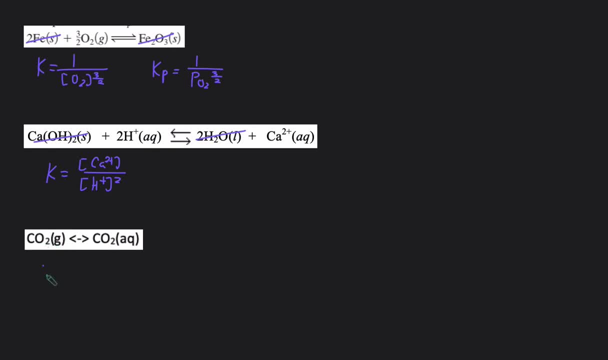 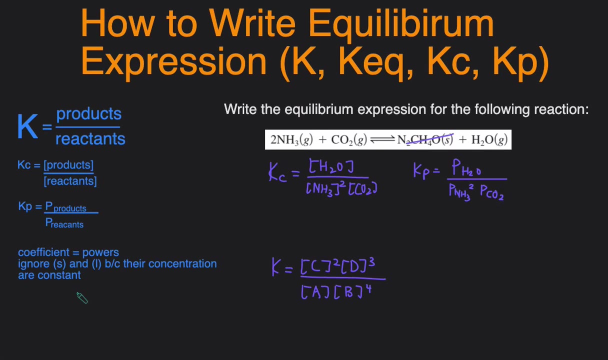 for aqueous and then use pressure when it's a gas. So our k expression would be the concentration of CO2 divided by the pressure of CO2. because this is aqueous, we use concentration, and then, because this one was a gas, we use pressure. And there you have it. that's how you would write the equilibrium. 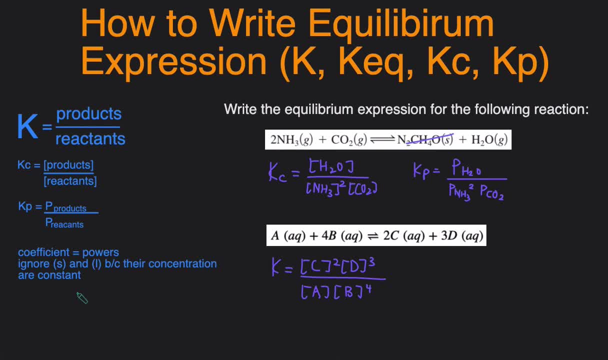 constant expression for any equation Reaction. so just to recap what we've learned: k is products divided by reactants. if it's kc, use concentration. if it's kp, use pressure. the coefficients in the reaction become the exponents in the expression and ignore solids and liquids because their concentrations are constant.